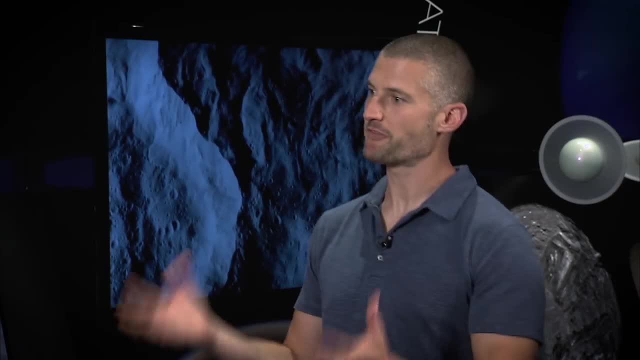 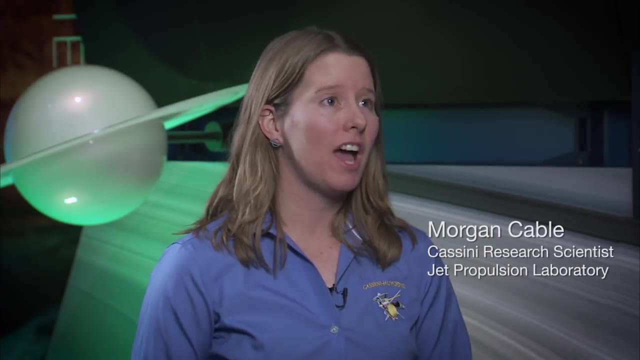 I am here with Morgan. She's a scientist on the Cassini project. The grand finale it's going to be 22 orbits about six months. What do we hope to accomplish in that amount of time? We hope to accomplish a lot of incredible science. 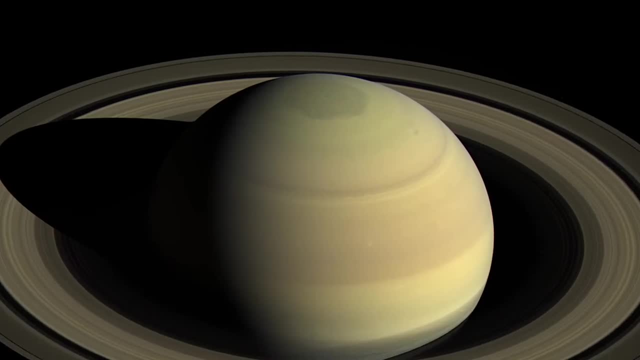 things that we have never been able to do before. with a Cassini mission, We're going to go screaming over the top of Saturn. We'll be able to study the Earth. We're going to be able to see the hexagon of Saturn's North Pole. 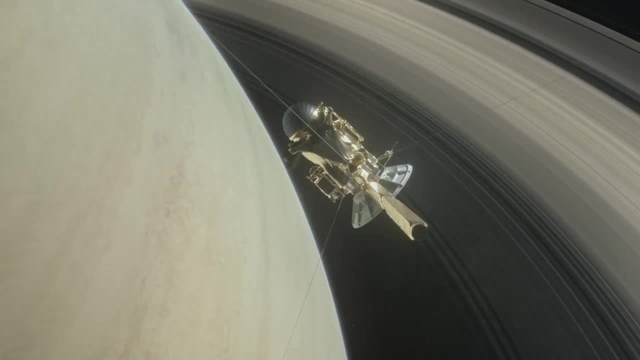 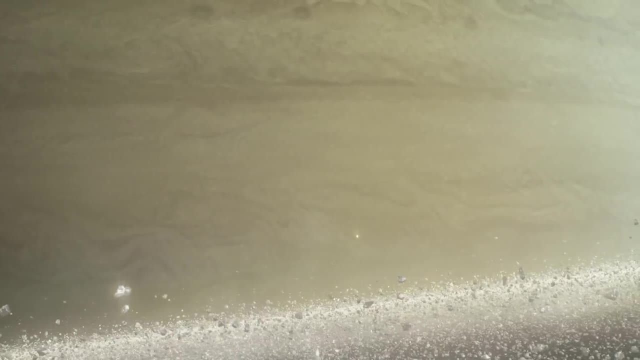 in greater detail than ever before. We're going to go shooting between Saturn and its rings, threading the needle, which means we'll be able to taste the ring particles, be able to understand more about what those are made of. We'll also be able to taste the atmosphere of Saturn. 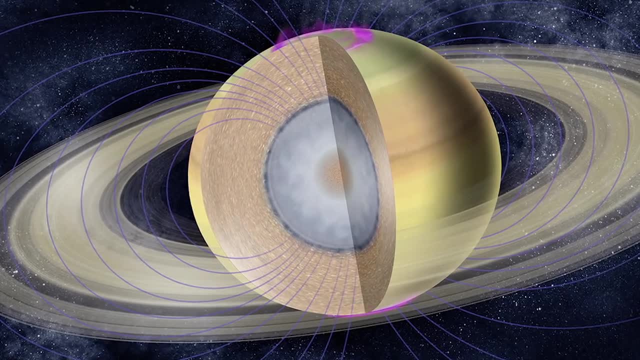 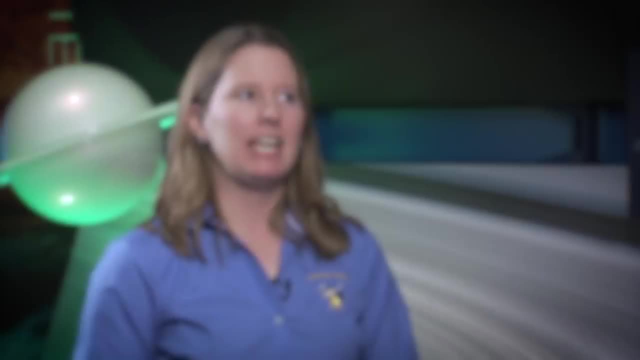 We're also going to get a better idea of the interior structure, since we'll be getting closer to Saturn than we've ever been, And then this will all culminate in Cassini's final plunge into Saturn's atmosphere, taking data for as long as possible. 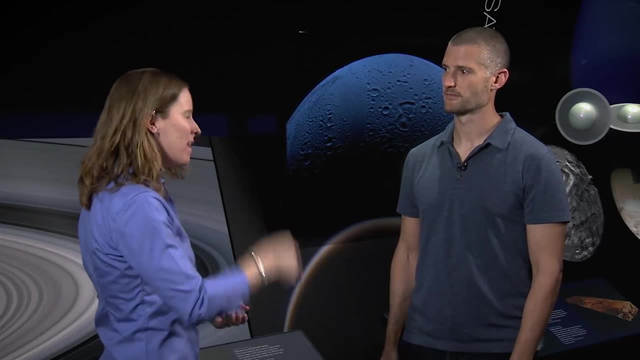 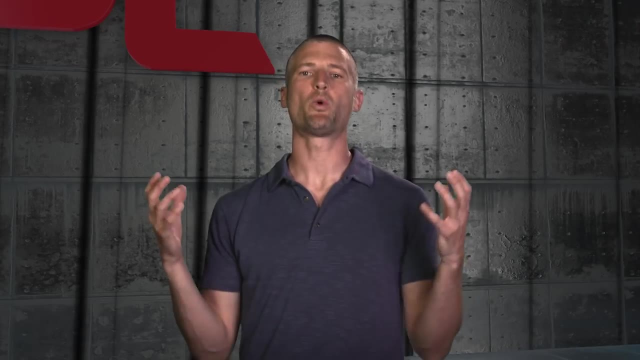 and sending that back to Earth. To be able to do this engineering, to thread that needle between Saturn and its rings- is really challenging. That requires something called astrodynamics. Okay, so what is astrodynamics? It's a form of engineering, but when we think about engineering typically, 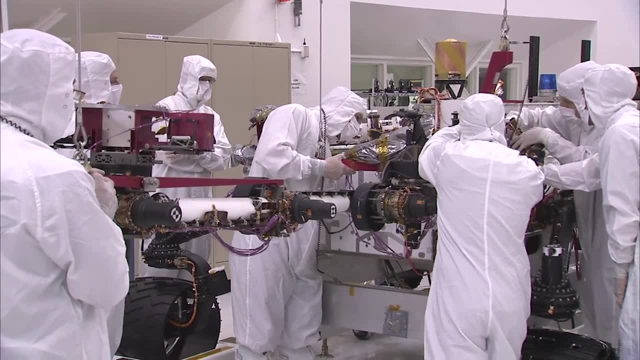 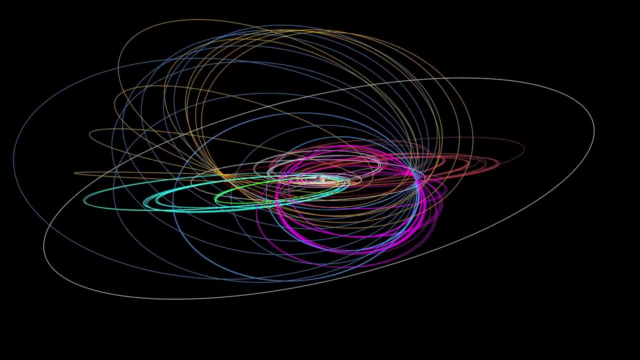 we think about people who are using physics and technology to build stuff. Astrodynamicists are building flight paths that will take our spacecraft to where they need to go. Let's go talk to one of the engineers who's pivotal in the design of this flight path on the Cassini spacecraft. 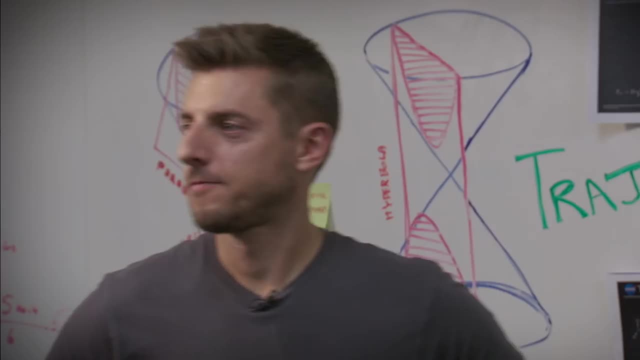 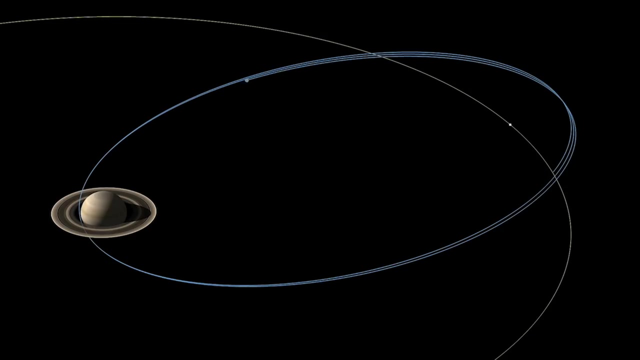 Okay, this is Brent. He's our astrodynamicist at JPL, Brent. what makes the Grand Finale particularly difficult and challenging? The Grand Finale is a series of 22 orbits where the periapsis, or the closest point of the orbit, 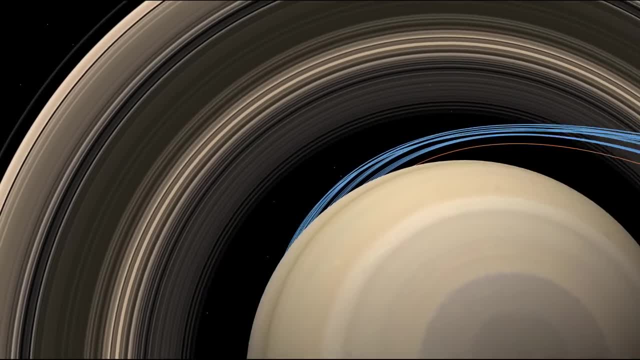 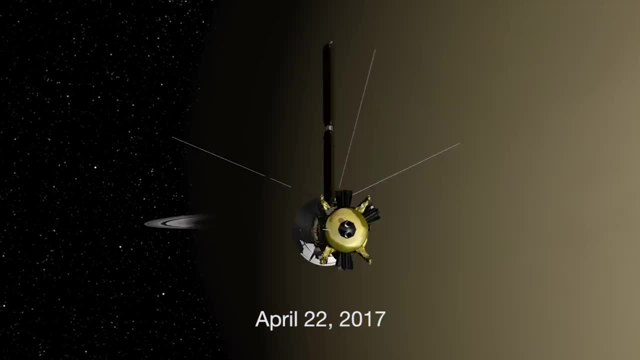 is actually in this gap between the upper atmosphere of Saturn and the innermost part of the main rings. What we've done is we've designed this trajectory such that, utilizing one last Titan gravity assist, we can jump the entire ring system and place the spacecraft orbit inside. 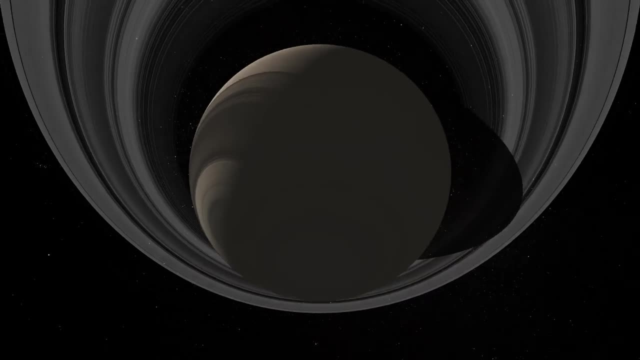 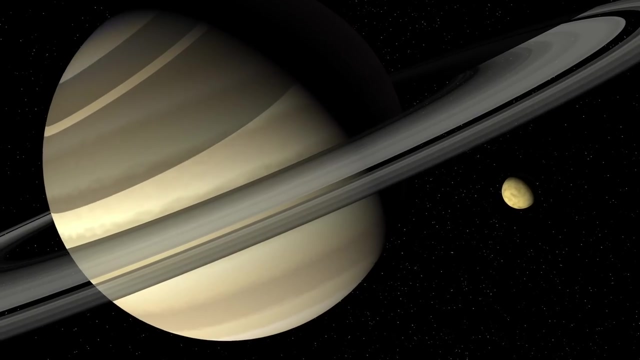 this very, very small gap that's only 2,000 kilometers wide. This concept of gravity assist. I think a lot of people have heard of it, but maybe not completely understand it. What it essentially means is you're harnessing the gravity of a body that's orbiting another body.